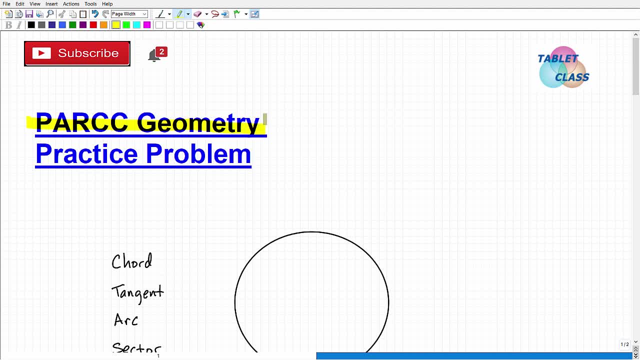 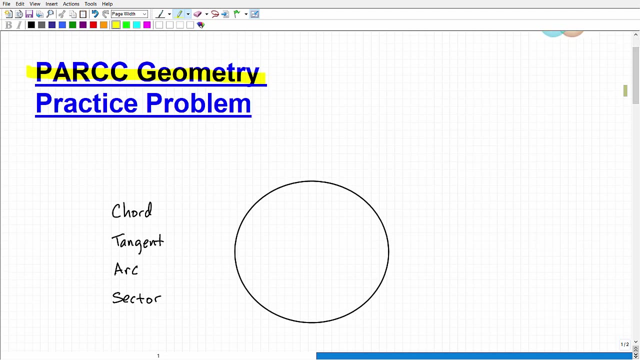 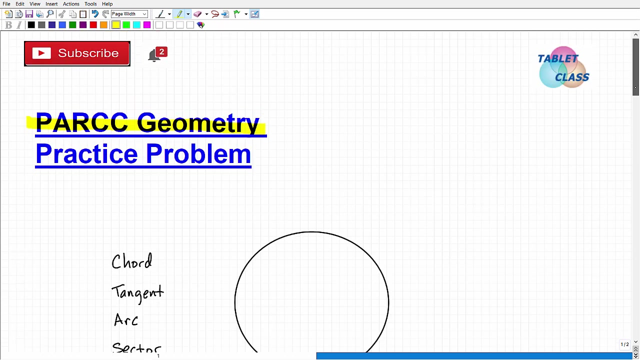 Park, Algebra 2.. So you're probably already familiar with the Park exam And by watching this video you obviously are preparing and taking it seriously. So congratulations on that. And what we're going to do here is take a look at a quick, a quick problem that hopefully you'll find pretty easy if you've done pretty well in geometry. Okay, but before we get going, let me go to introduce myself. My name is John. I'm the founder of Taba Class Math. 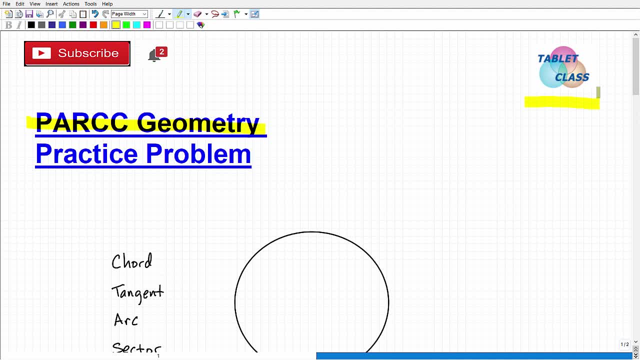 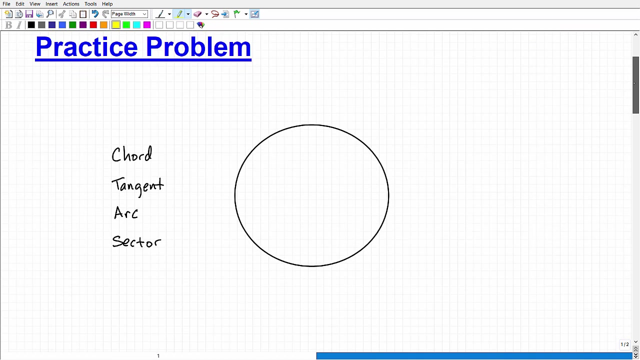 I'm also a middle and high school math teacher And over several years, I've constructed many, many online math courses to include a Park Geometry test prep course. I'm going to leave a link to that in the description of this video: Really comprehensive course. If you feel like you need some additional assistance in preparing for the Park Geometry test, Okay. so with that being said, let's go ahead and take a look at my little pop quiz here Now. geometry is a huge topic. Circles are very, very important. 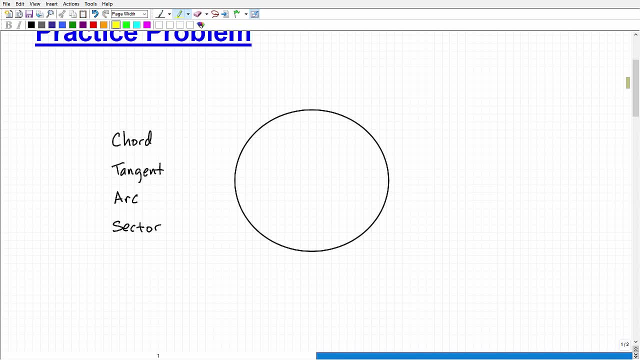 And in geometry. before I get to this problem, you know we learn a lot of things like- and I mean let's just kind of quickly talk about some of the things that you've learned- right, Well, you learn a lot of postulates, you learn a lot of theorems, a lot of properties, a lot of definitions, And you know all of this. I mean, if you think about it, if you look at your, your notebook, you know you have, you know, probably likely, you know a couple of things. 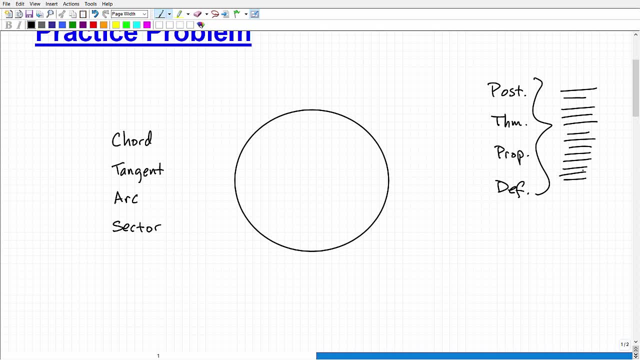 A couple hundred pages full of all these formal definitions, postulates and theorems and everything else that you've written down. Now I don't think you know any teacher expects you to. you know, use flashcards and use your rote memory to just remember all this stuff you know by. you know perfectly, you know recall every single theorem, every single property, etc. 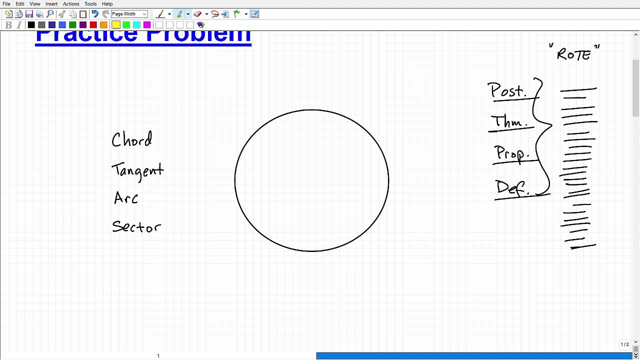 I don't think that's the you know really the spirit of what you're trying, We're trying to do as teachers in geometry. However, what you do need to have is a firm grasp on the concepts, OK what these things are communicating, these postulates and theorems, even if you recall them perfectly. you need to understand them. 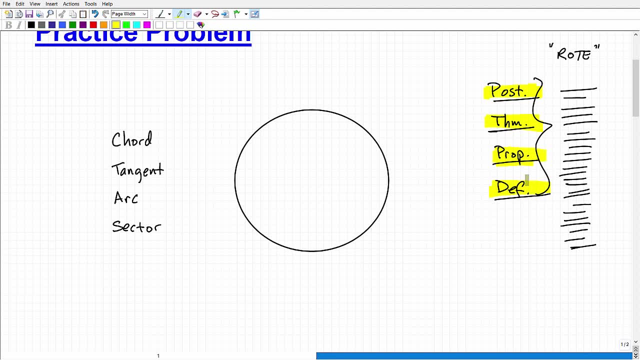 OK, there is a lot. So that is, I think, how you want to approach it. But again, you know you want to check with your teacher and see what kind of guidance that you're kind of given. But there are. you know, I think for most students they get kind of overwhelmed with just 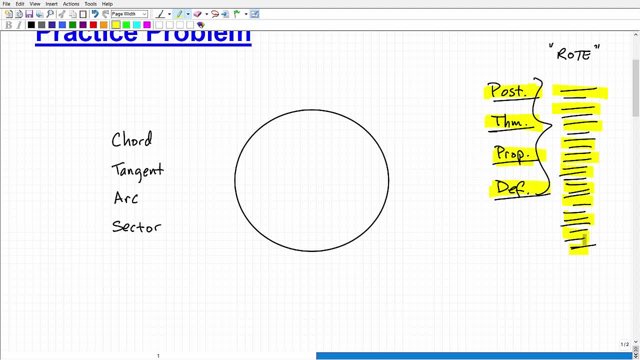 I'm trying to memorize all this stuff, Don't worry about it. However, OK, when it comes to definitions, you do have to have a pretty good grasp on. you know terms. OK, we're talking about various things, So, again, you don't have to know them perfectly, but you do have to know what we're talking about. 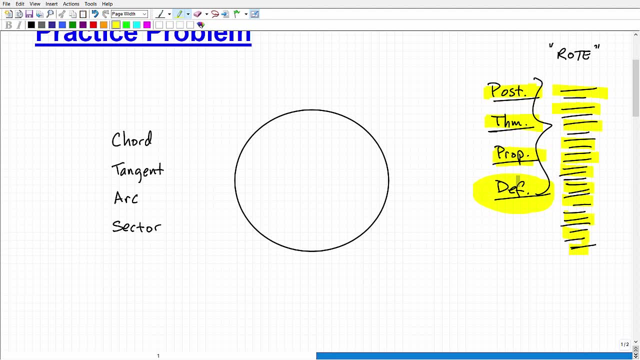 So that leads me to my little pop quiz here. So we have a circle and I have some words, OK, so chord being one of them, Tangent, OK being another arc and sector, OK. so just want you to think about it real quick and see if you remember the definitions. 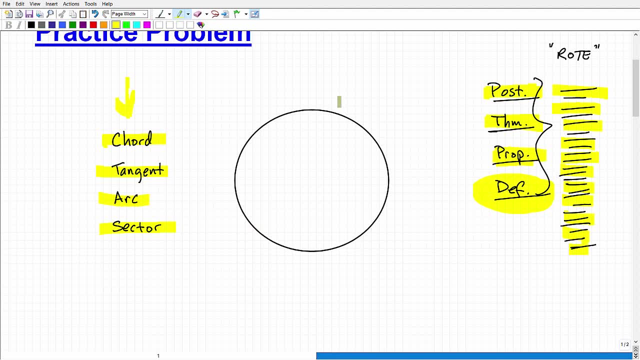 OK, you certainly know the words when it applies to, when it comes to a circle, But what are they? OK, make sure you specifically know And I wouldn't suggest you know going and looking, you know in your notes or just you know. take a quick moment, pause the video. 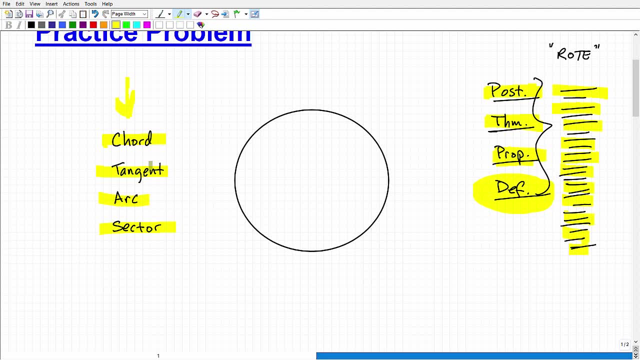 And think about: hey, do you know what a chord is, A tangent, an arc, a sector? OK, there's other things I could throw in there, But let's just use these, because these are generally kind of new definitions in high school geometry. 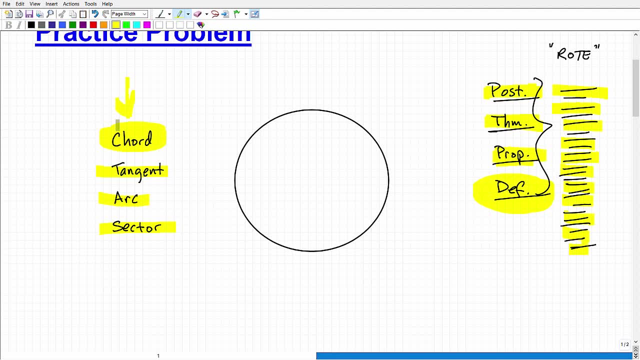 OK, so let's talk about a chord. OK, so a chord is what? Well, it's just a line, OK, that goes from one end to the circle to another. All right, So I can have a chord like. so I can have another chord like, like this way: 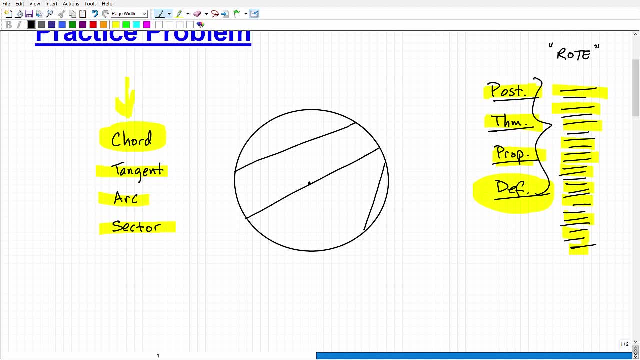 And then, of course, I can have a chord that goes through the center and hopefully you'll say, oh yeah, by definition that is the diameter. OK, so this is a chord. Now chords do not continue on like so. 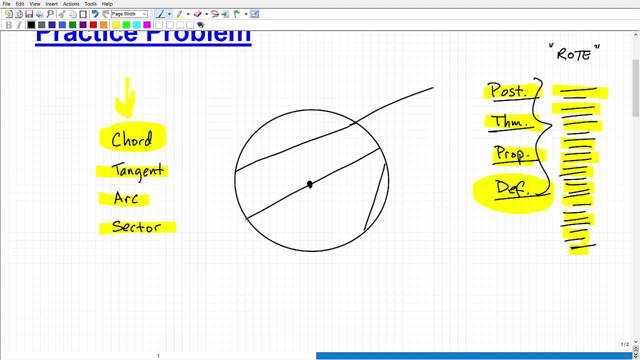 OK, they do end from one side of the circle to the other. OK, so that's the basic concept behind a chord. OK, how about tangent? Well, that word tangent And we can kind of think of in terms of a tangent line. 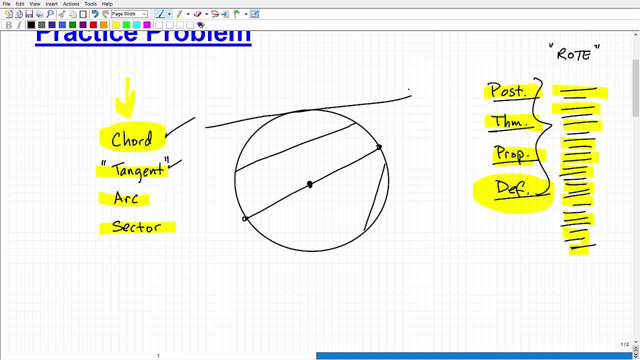 Right. So the concept of a tangent, and we kind of draw a little line like so, All right. So let's say this line is just barely touching this circle and it's going to be. that's a line that's tangent to the circle. 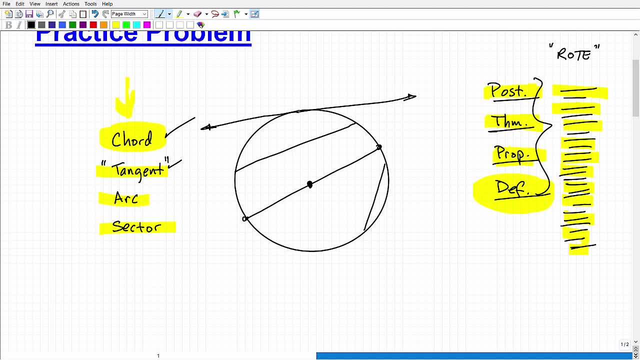 That's what that means. So this is a tangent line and this is the point of tangency. OK, so it's touching the circle at one point, Point OK. so that's the concept of tangent. OK, so hopefully you're doing pretty good with this. 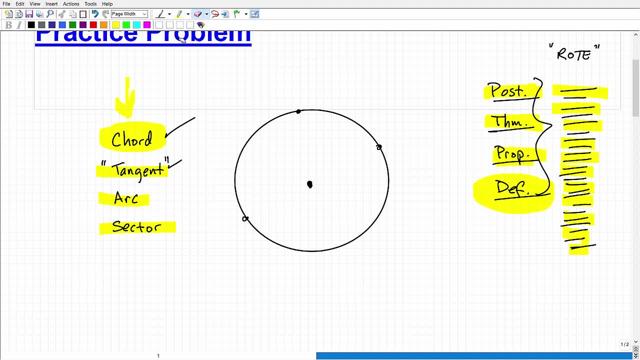 Again, this shouldn't be too difficult, but again, we don't want to confuse ourself with terminology. OK, remember, you know a lot of these postulates and theorems and properties and stuff. You know- I'm not saying, by the way, you don't need to try to remember all this stuff- pretty well, 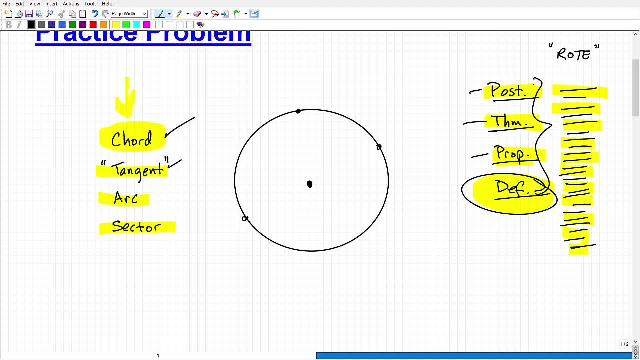 OK, I'm just saying it's not going to be perfect, But you do have to have the Gist of the meaning and it has to be accurate, All right, So let's go in and take a look at our next word here. 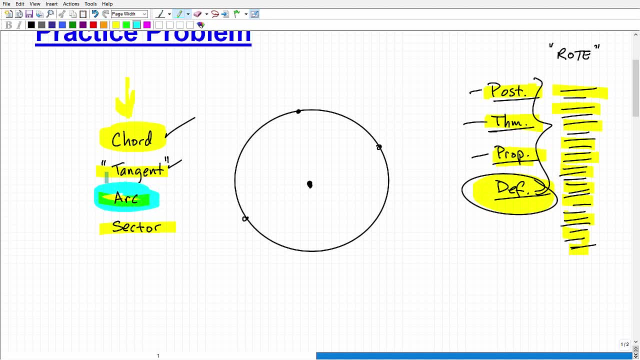 And that's an arc. So what is an arc? Well, an arc is a measurement that goes along the out some portion of the circle, OK, like so. OK, And we measure that in degrees. So this might be, for example, a 60 degree arc. 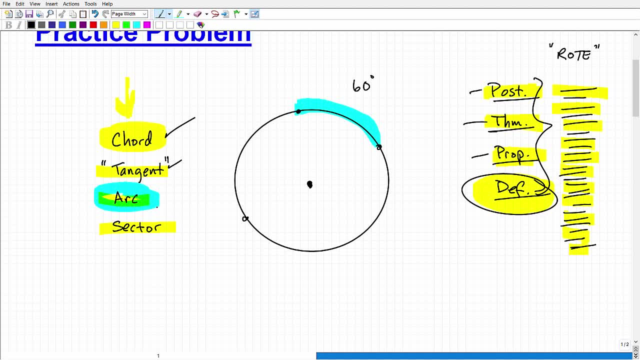 Now, along with that, you're going to need to know the various Notation that goes into that. All right, So we can kind of look at it like: so, This is an arc, And then that leads us to our last word, sector. 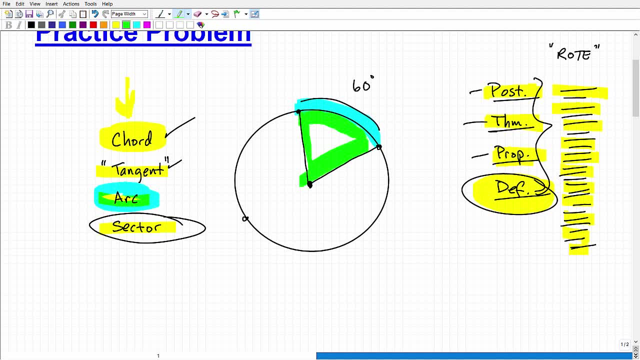 OK, And hopefully you knew that. Oh, this little pizza slice like this is a sector OK, This is a sector OK, And this is an arc. You don't want to confuse those two, All right, OK. So I think, on the scale of you know, one being easy and ten being hard, this is like maybe a level. 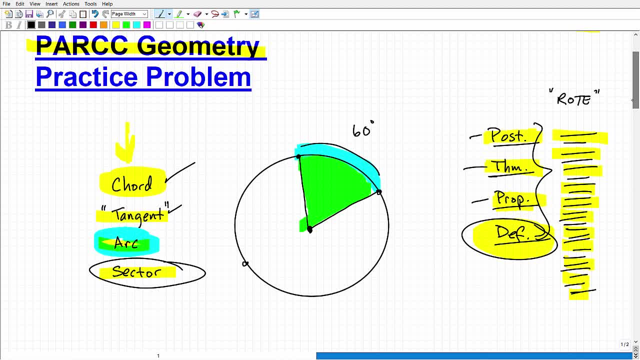 Three problem: OK, Real basic, foundational stuff. But you know, as teachers, I'm not surprised that a lot of students still struggle with the fundamentals. OK, So, again, you know, if you're studying, there is time for you to you know, relearn this stuff. 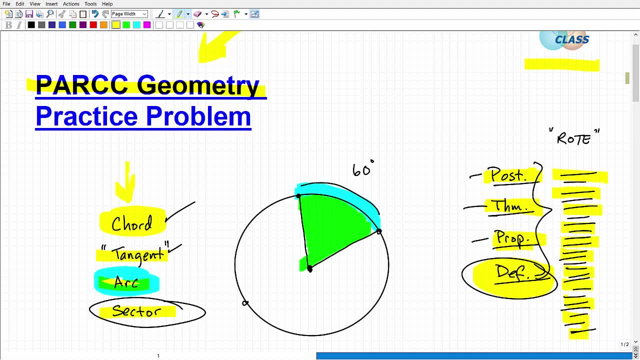 You don't want to go in to this park geometry exam, you know, and you know basically already, knowing that you're struggling with concepts. OK, If you have time to do something about it, study really hard, Because all this stuff is important. 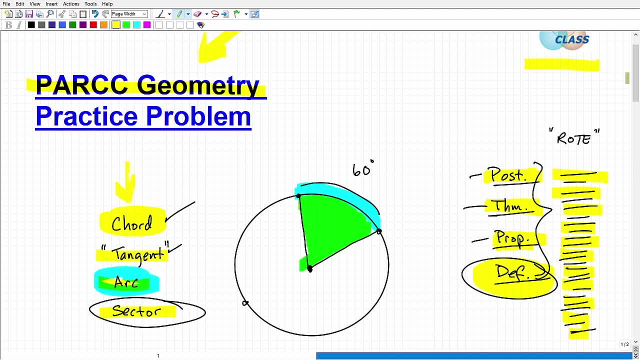 Your whole high school education is critical. OK, Geometry is a very, very important topic. OK, Where is geometry going to come up in your future? Well, you're going to see these concepts play out, Some of them in algebra two and pre-calculus. 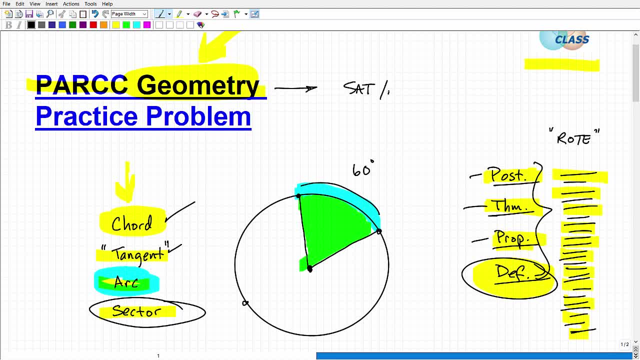 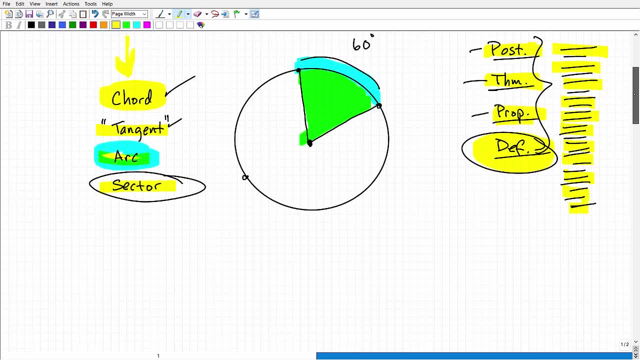 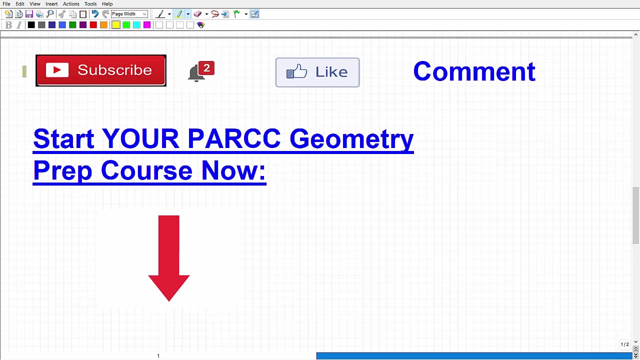 But, just as importantly, a lot of tests like SAT, ACT, entrance exams, CLEP exams, et cetera. So it's all important, OK, So let's go and wrap up this Video. So, on the time at the time I made this video, I've been on YouTube for a good 12 years. 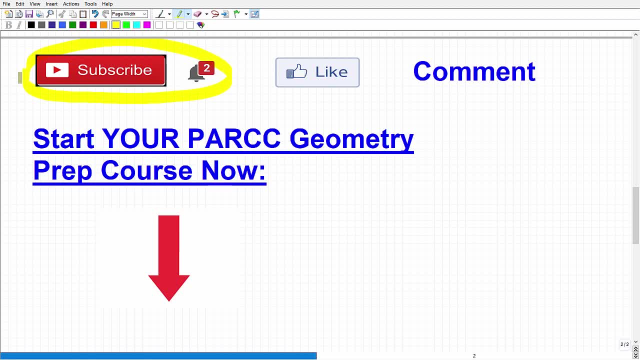 I have hundreds of math videos. If you like my teaching style. we have a lot of stuff on my channel that can help you out, And I'm posting new stuff all the time, So hopefully you'll consider subscribing If you enjoyed the video. definitely appreciate a thumbs up and leave me some feedback. 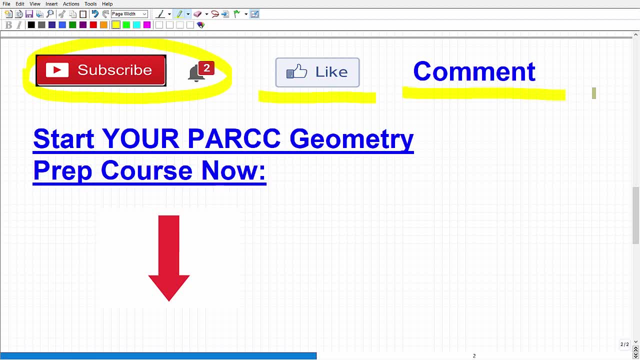 How do you like geometry? I tend to find students either like it or they don't like it. You know a lot of students like algebra, They don't Like geometry, or they like algebra and geometry. But geometry is a different. you know subject altogether. 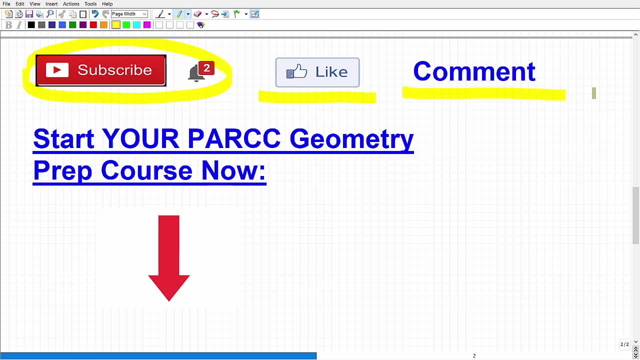 One thing that makes geometry unique too, I think a lot where a lot of students don't like geometry is this idea of proof Right, The postulates, the theorems and, you know, proving stuff and writing those proofs- that that is difficult for most students to kind of grasp. 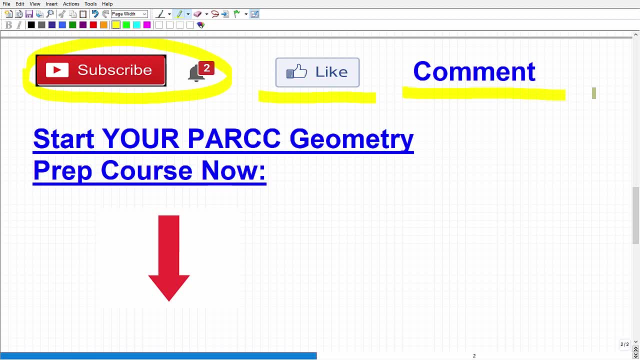 OK, but that's really when you're learning there. It's kind of like a real essence of more advanced mathematics. So, again, all important stuff, But anyways, it means the feedback. Let me know how geometry went for you, And then, as a reminder, I'm going to leave a link to my park geometry test prep course in a description of this video. 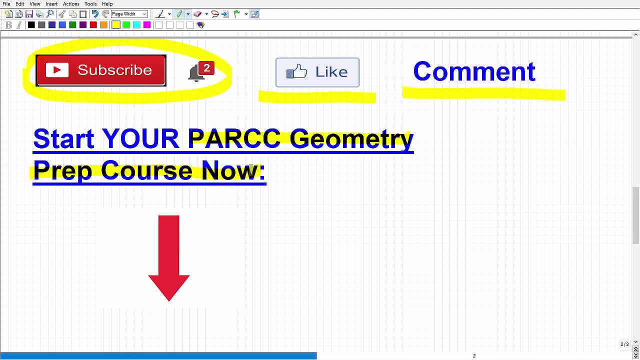 It's super, super comprehensive. It's effectively a full on geometry course and will definitely help you out on a park, But always like to leave students with this. Always listen to your teacher first. Take advantage of everything that the school and your teacher is giving you with respect to the park test prep. you know preparations. 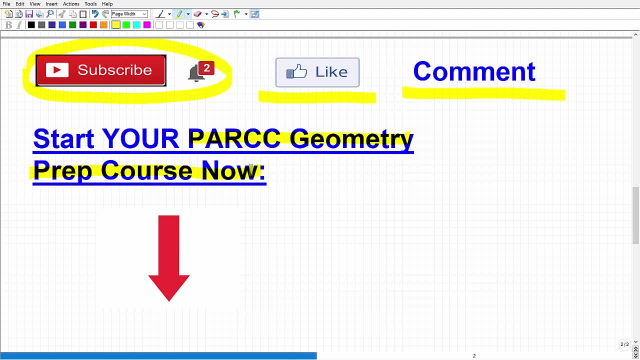 OK, but if you feel like you need something above and beyond that, then a course like mine could serve you well, OK. so, with that being said, thank you for your time and have a great day. 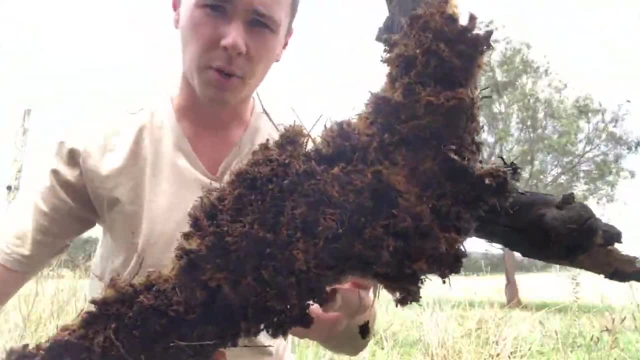 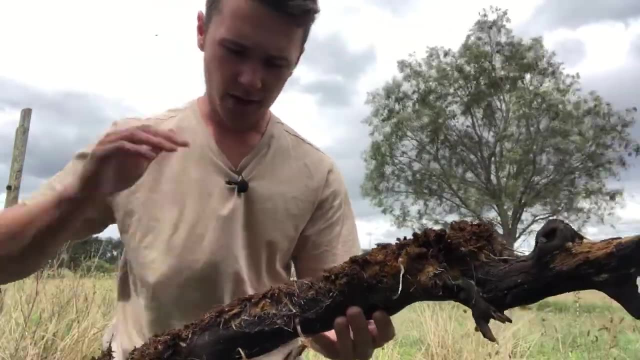 So you may be able to see here all of this yellowy, brown kind of stuff attached to this piece of wood, But what it actually is is fungi. So that's exactly what we'll be talking about today in this video, And we'll be looking. 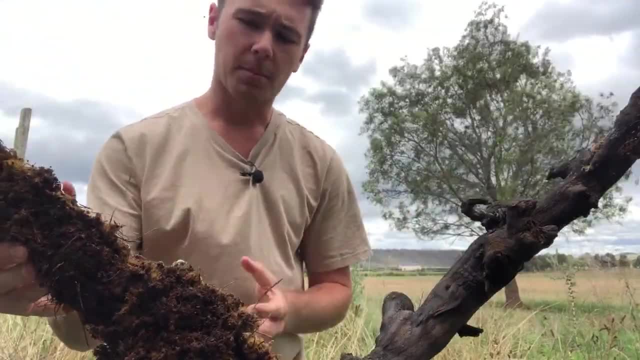 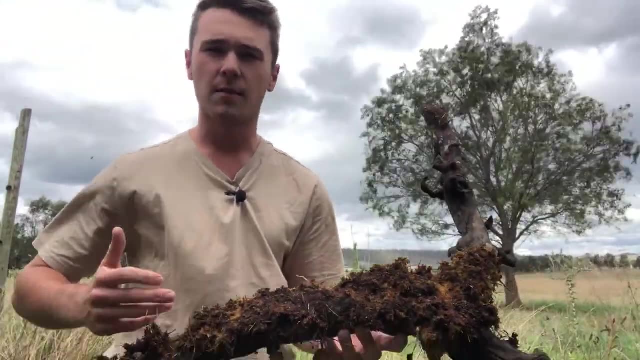 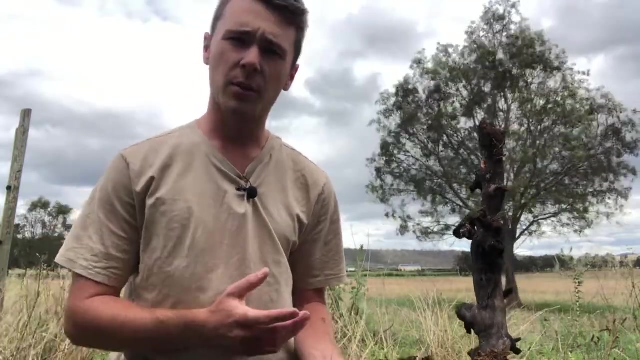 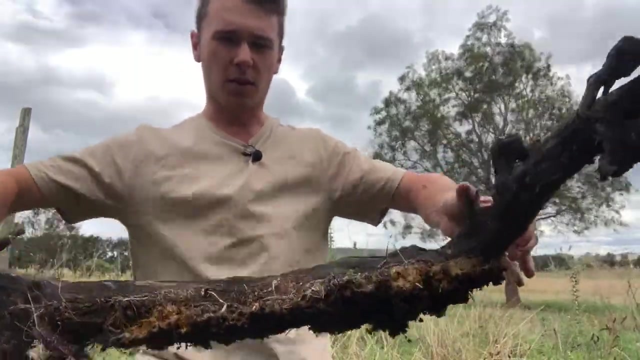 at how this fungi breaks down pieces of pretty much woody material and returns it to either soil, organic matter or into the fungi biomass itself. We'll be talking about the benefit that brings to our soil and our farm and how we can also increase the fungi on our farms. So you can see here the piece of wood was. 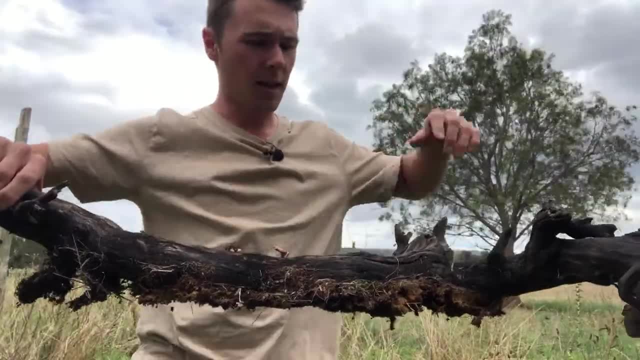 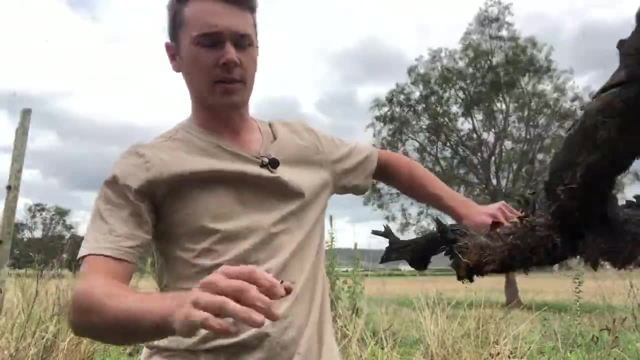 lying down like that. So it had contact with the ground from underneath and pretty much it's starting to break down the woody mass from underneath And you'll also be able to see on this side the fruiting body of the fungus on the wood. 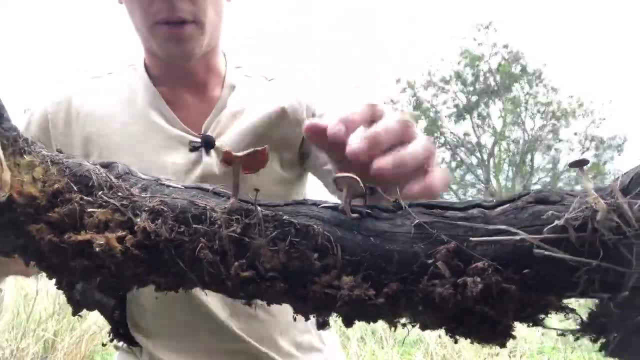 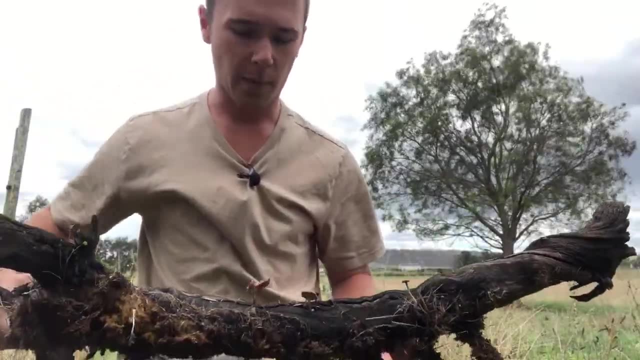 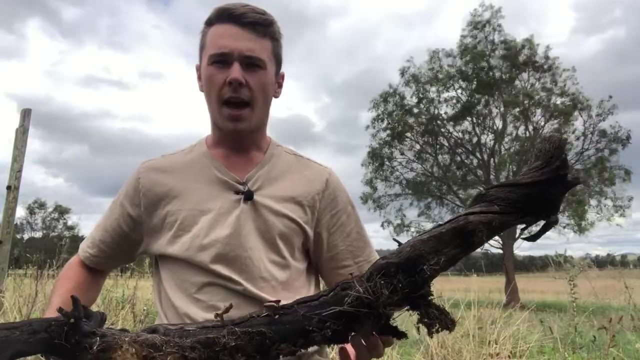 just here. So that's actually the fruiting body. The fungi would be spread all across, all within this piece of wood and be actually decomposing it from the inside and from the bottom. Anyway, stay tuned to see the whole video. My name is. 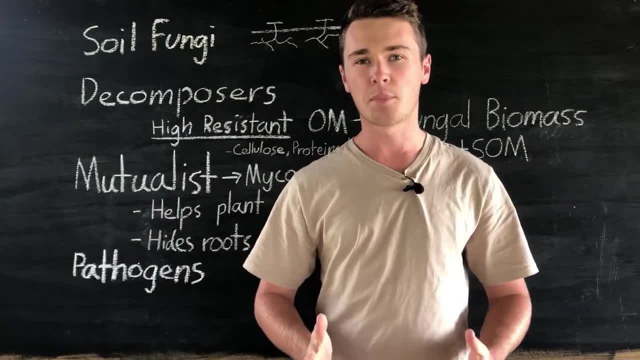 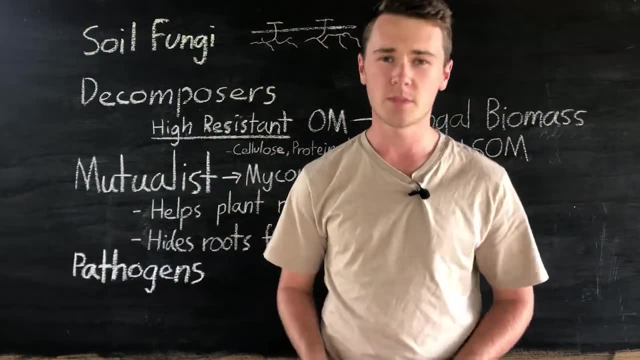 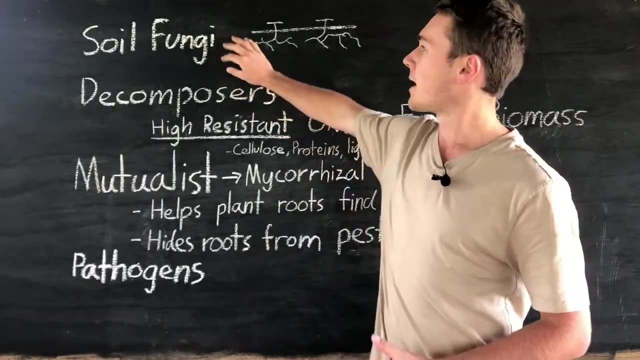 Teal Simmons, and this is Agriculture Explained. One of the most important microbes in our soil are soil fungi. So fungi are a group of organisms that are different to plants, animals, bacteria. They're a totally different group of organisms. Now, fungi are: